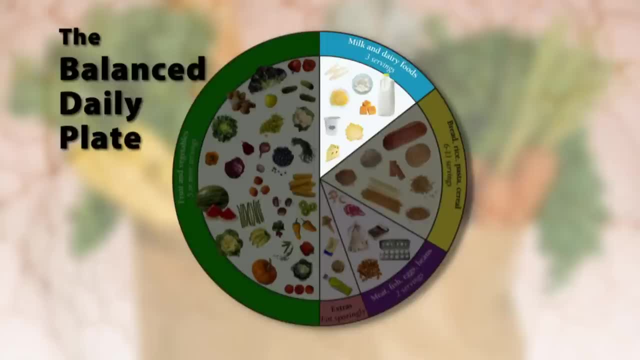 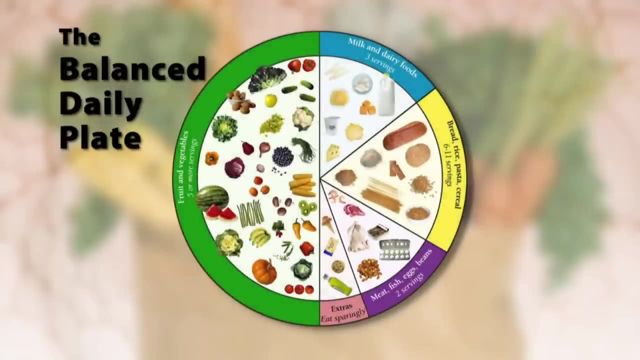 We also need to eat some dairy foods, such as low-fat milk or yogurt, as well as lean meat, fish, eggs or beans. We don't need to eat all the foods shown in each section at every meal, or even every day, but we do need to eat some food from each of these groups. 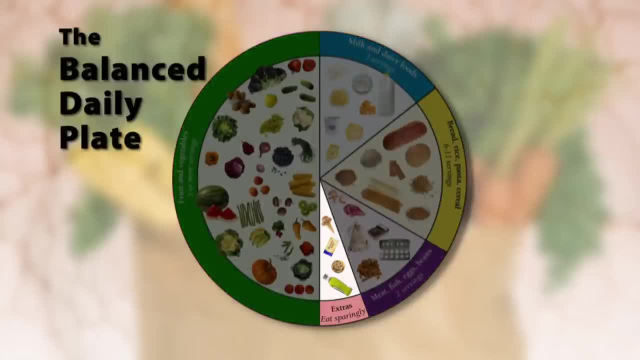 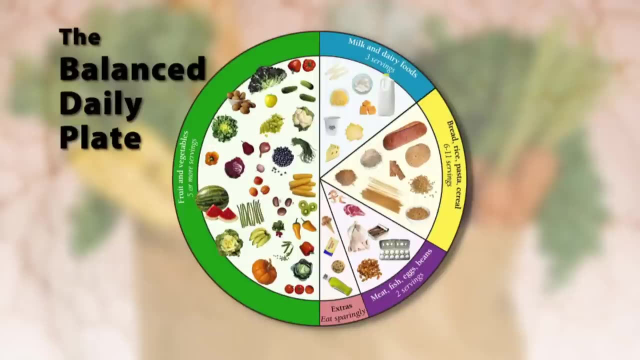 We can eat a lot throughout the day, the exception being the extras group, of course. We don't need to eat anything from this group every day, or at all. Everything we eat during the course of the day at meals and snacks, as well as the things 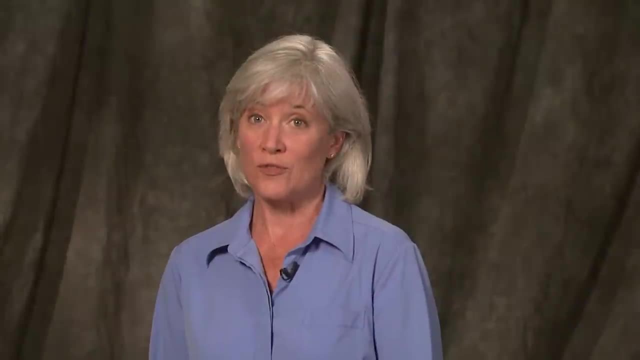 we drink should come from these food groups. Each group includes foods that are similar because they have comparable amounts of the same nutrients. For example, if I plan to eat cereal for breakfast but I discover I don't have any cereal, I 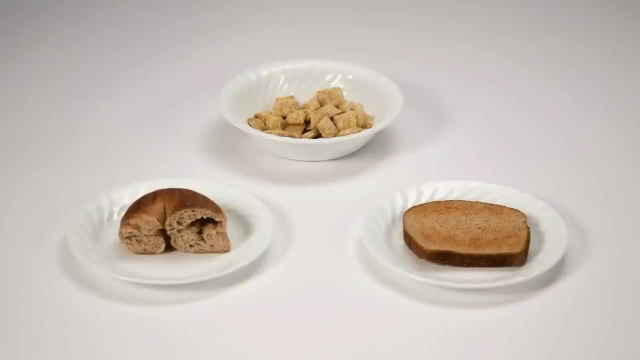 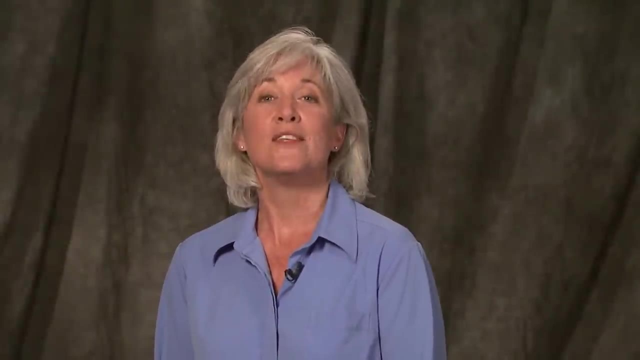 know I can choose something else from that group. We can also choose to eat a half-meal meal, like a toast or half a bagel, and still get the same nutrients. This also helps honor the food preferences of individuals you support. 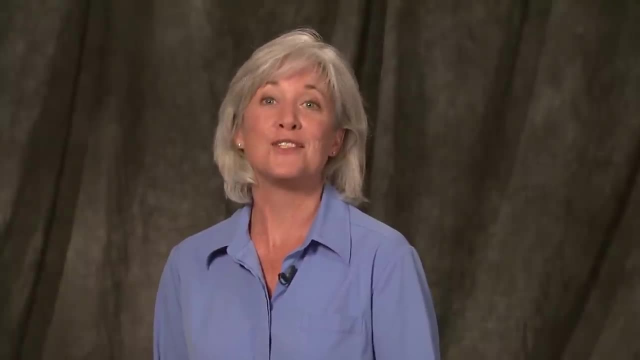 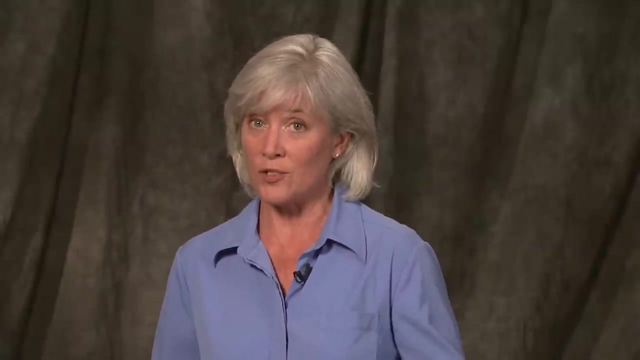 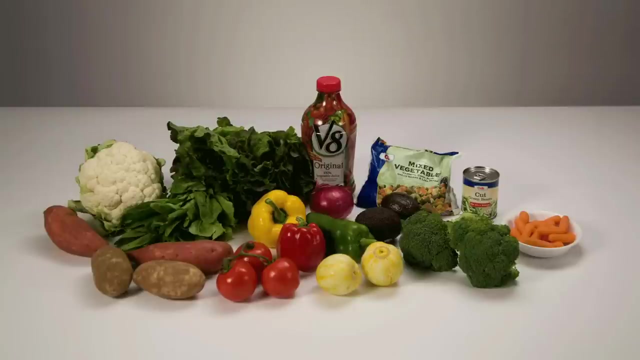 This way, everyone in the home can choose what they want to eat and still get the nutrients they need. Now let's talk about each of the groups individually, starting with vegetables and fruits. The vegetable group includes any vegetable, whether fresh, frozen, canned or dried, or 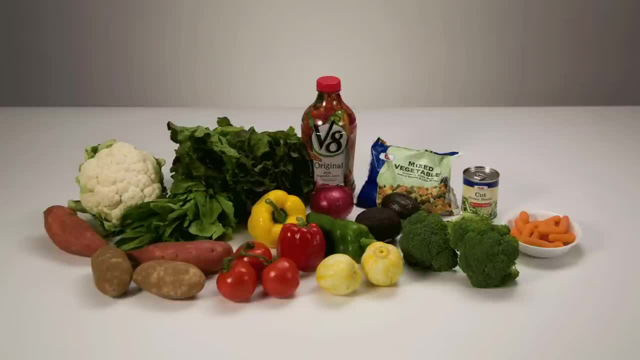 100% vegetable juice. There's such a wide variety of vegetables, each with its own unique taste and texture, from leafy greens like romaine and leaf lettuce to root vegetables like potatoes and carrots. Vegetables provide us with a wealth of nutrition. 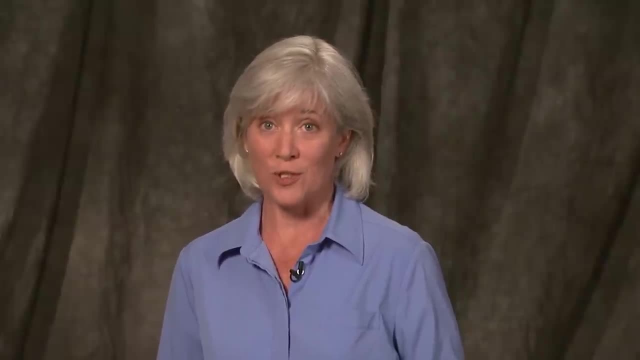 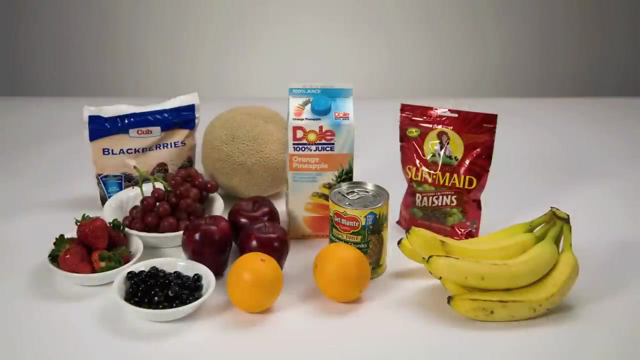 For juice, the label must say 100% vegetable juice to count as a serving of vegetables. The fruit group includes any fruit or 100% fruit juice. Juice may be fresh, frozen, canned or dried. Examples include raspberries, strawberries, blueberries, blackberries, melons, oranges. 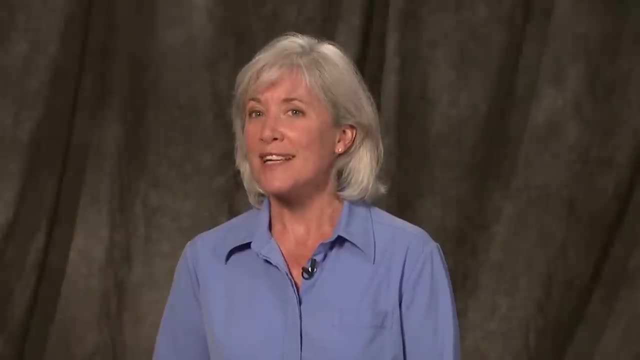 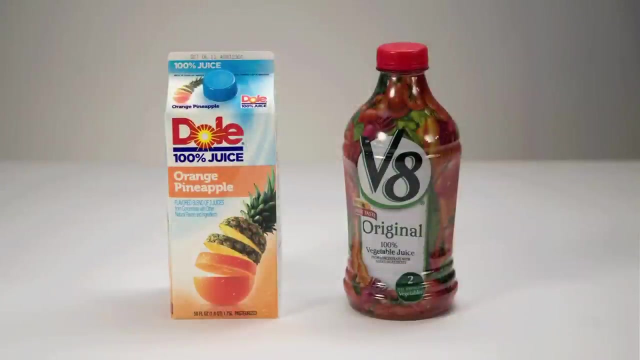 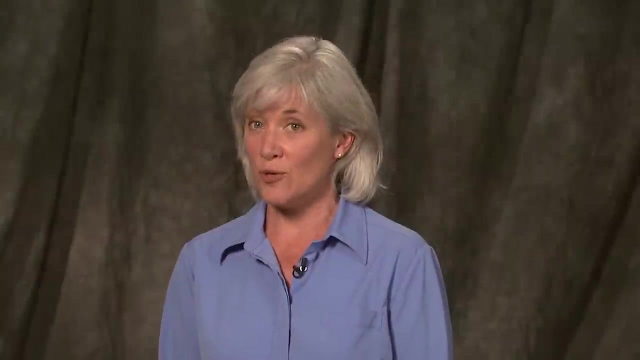 apples, bananas and grapefruit. There are just a couple of things to remember about canned fruits and fruit juice. Just like with vegetables, for a juice to count as a serving of fruit, the label must say 100% fruit juice, Labels that say juice drink or any drink that is labeled as. 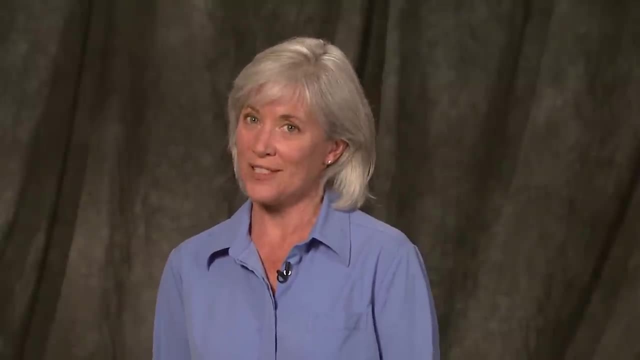 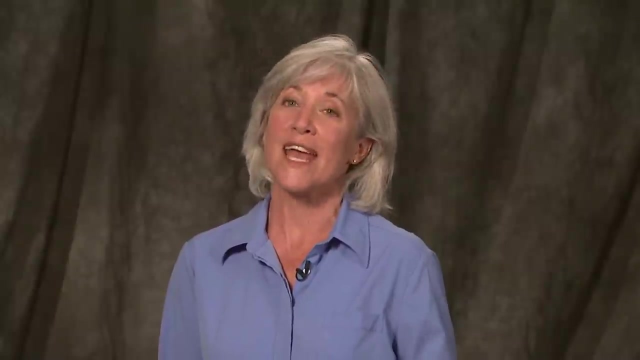 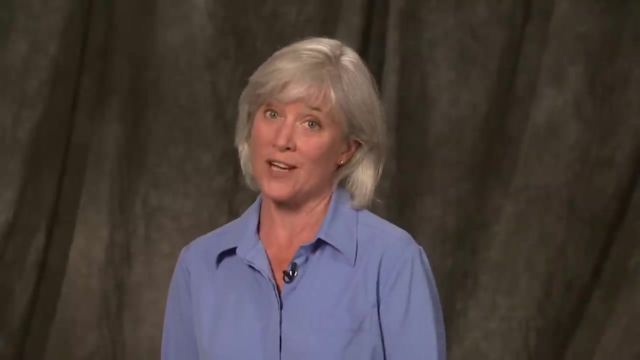 local fruit may be fresh, frozen, canned or dried. Also, look for fruits that are canned in juice. Fruits canned in juice do not have any added sugar, But fruits canned in syrup, whether it's light or heavy, do have a lot of sugar added. 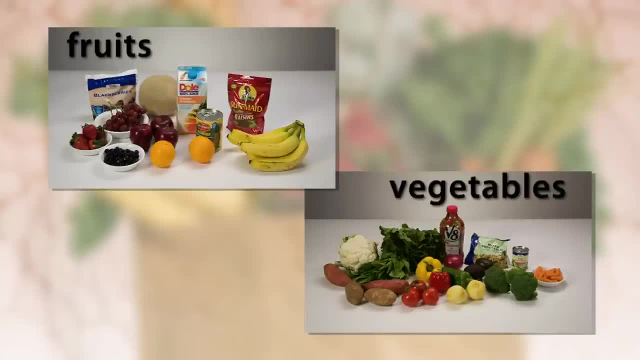 Most people need to eat at least five or more servings of fruits and vegetables each day. You could pick any five and you'd be getting enough nutrients from this group that you need for the day. Now let's talk about the grain group. 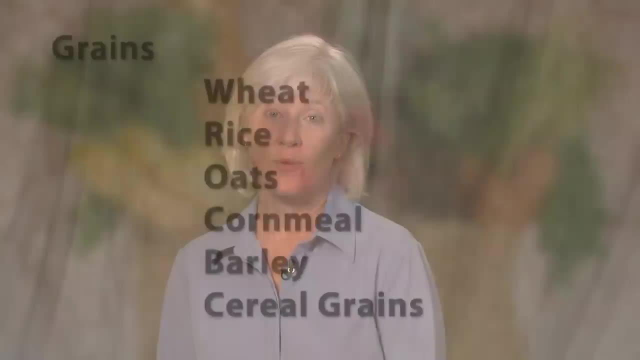 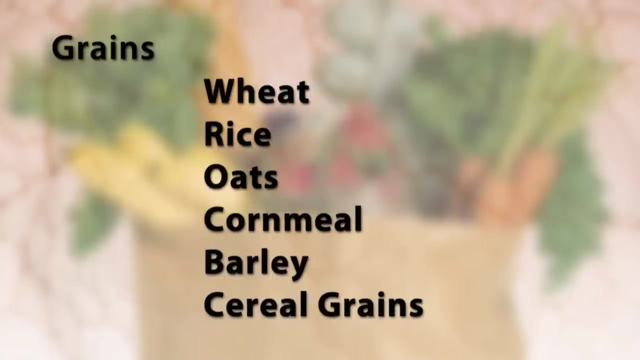 Grains are also one of the foundations of a well-balanced diet. We use wheat, rice, oats, cornmeal, barley or other cereal grains to make some of the foods in this group, which include bread, ready-to-eat cereals and cooked cereals. 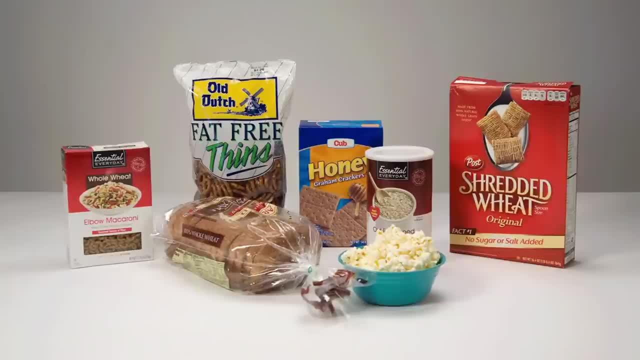 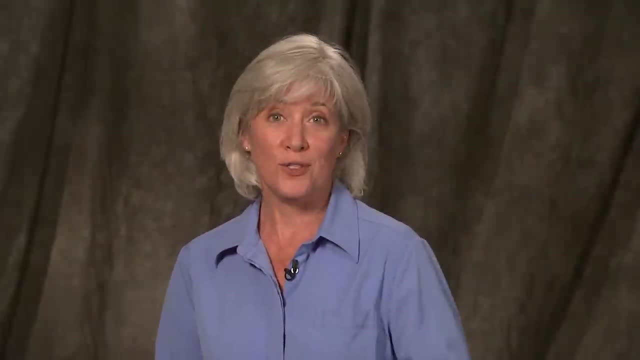 Other grain foods include pasta products, pancakes, rice, tortillas, graham crackers, saltines, popcorn and pretzels. The grain group also includes foods that are newer to some of us, such as quinoa, frica, amaranth barley and wild rice. 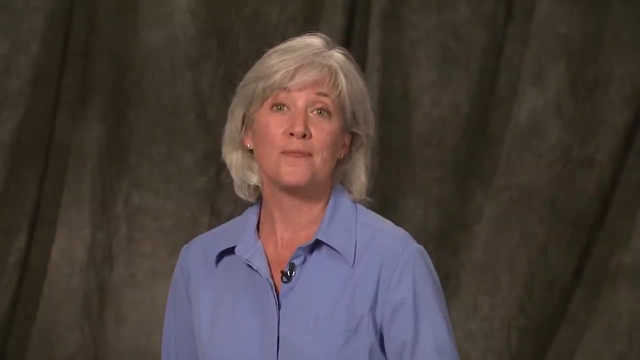 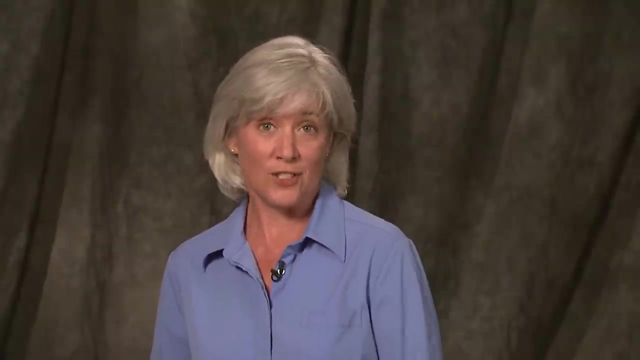 Perhaps some of you or your staff have used some of these foods before. These grain products are rich sources of nutrition and can be incorporated into tasty dishes that everyone can enjoy. Everyone needs a minimum of six servings each day, but some people need up to 11 servings. Individuals who are less active need fewer servings. The grain group also includes foods that are newer to some of us, such as quinoa, frica, amaranth barley and wild rice. Perhaps some of you or your staff have used some of these foods before. 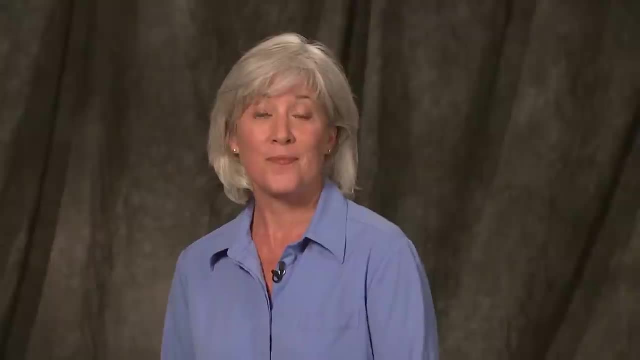 Individuals who are less active need fewer servings, while those who are very active need more. Try to make at least half of your grains whole grains, like 100% whole wheat bread and pasta or brown rice. We'll talk more about whole grains in the next session. 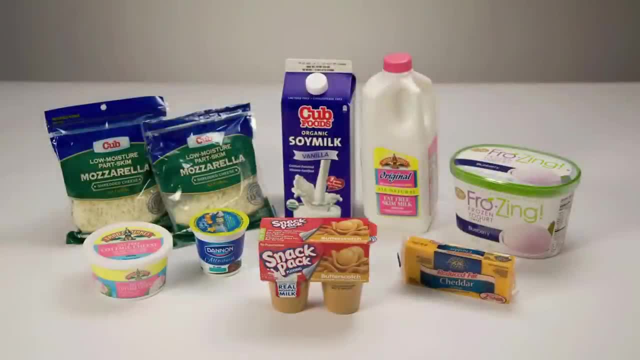 Let's leave grains and move on to dairy foods. Dairy foods are generally made from the milk from cows, goats or other animals. Fortified soy milk is also considered to be in the dairy group, even though it's not from an animal. 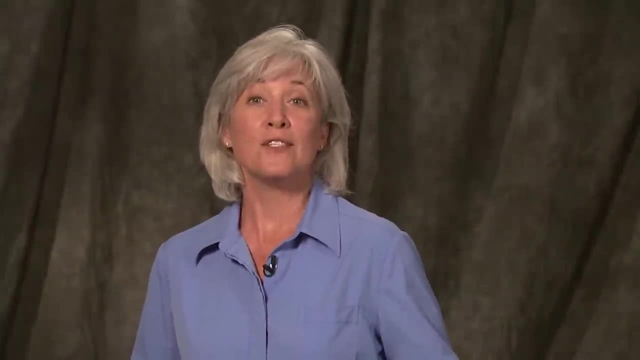 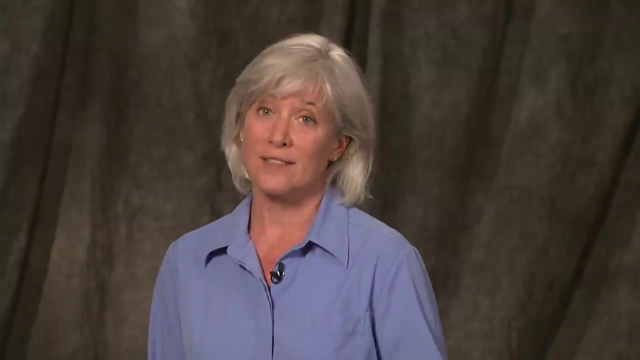 Dairy products are a very important part of the daily diet and are the best source of calcium and vitamin D. Dairy products aren't only important for growing children. they are just as important for adults. Even though we have reached adulthood, we still need to have three servings from the. 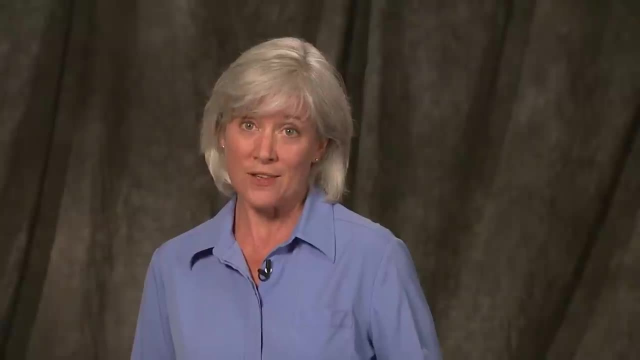 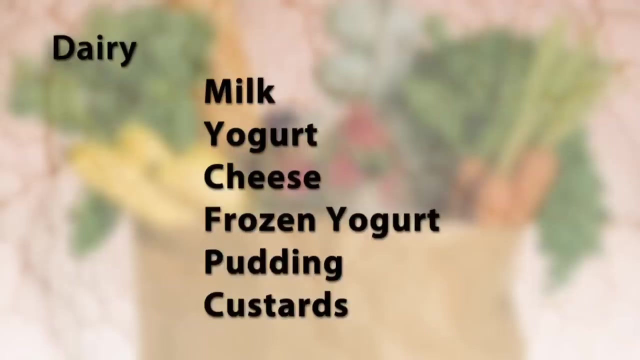 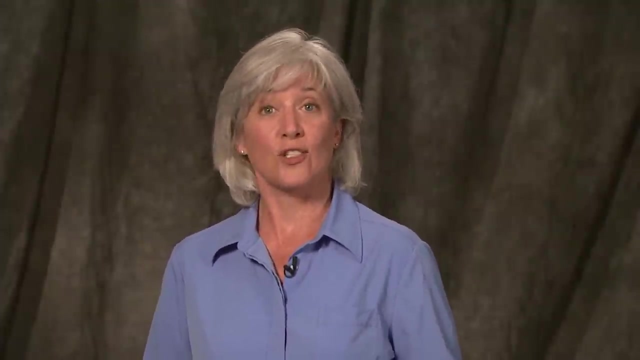 dairy group every day to make sure our bones and teeth stay strong. The dairy group includes milk, yogurt, cheese and milk-based desserts such as frozen yogurt, pudding and custards. Combination foods made from milk and milk products such as cream soups and macaroni. 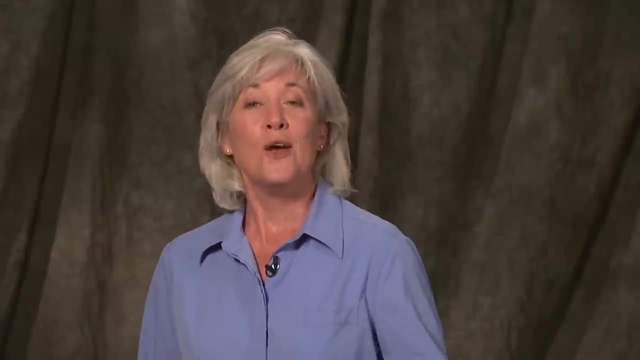 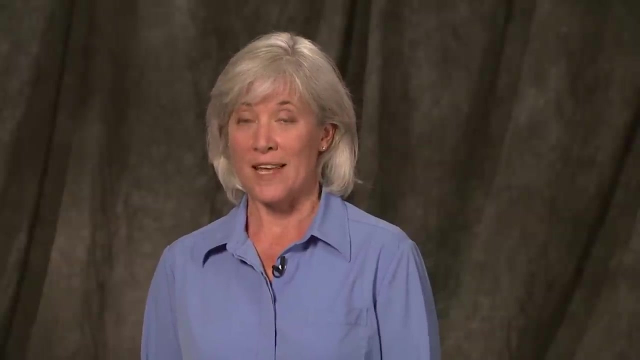 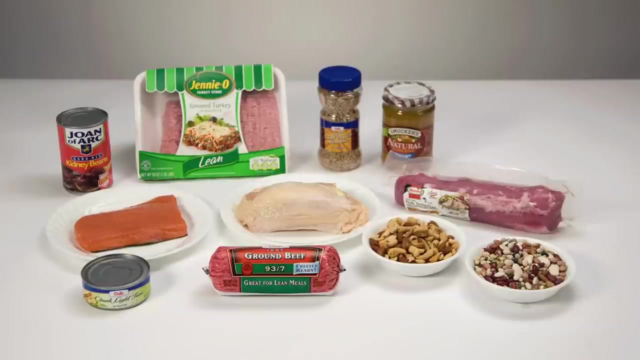 and cheese also contribute to the dairy group. We'll talk more about combination foods later in this session. The last food group we'll talk about today is the protein group. The foods in this group are valuable sources of protein, iron and B vitamins. 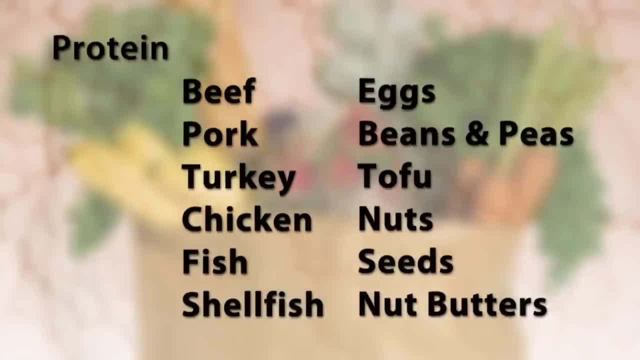 The protein group includes beef, pork, turkey chicken and vegetables. Don't forget to subscribe to our channel for more videos on protein. yogurt, cheese and dairy fish, shellfish, eggs, dried beans and peas, tofu nuts. 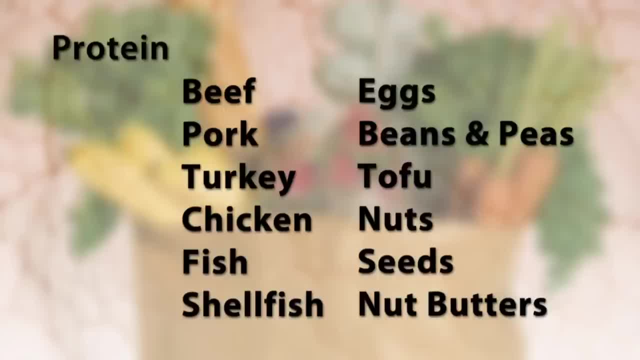 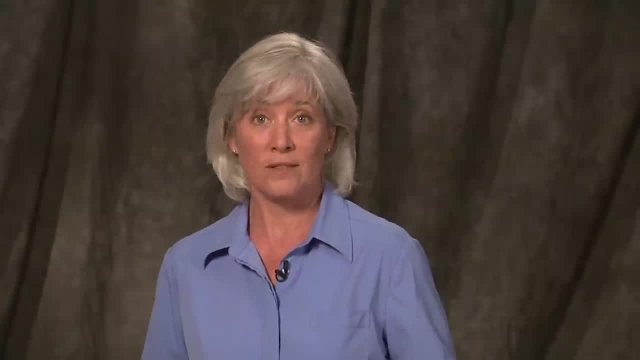 seeds and nut butters such as peanut or almond butter. Protein also includes other animal products that are served in a variety of cultures, such as goat, lamb, rabbit, venison, duck and pheasant. If we eat protein foods twice each day, 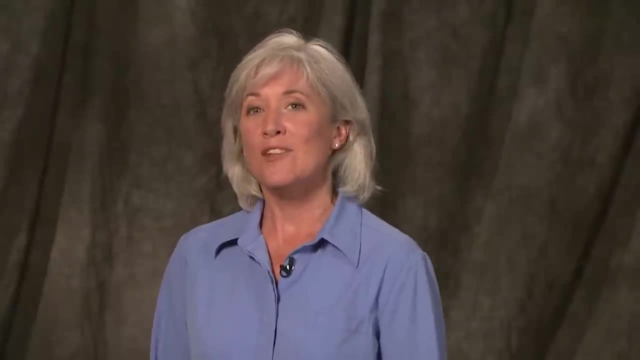 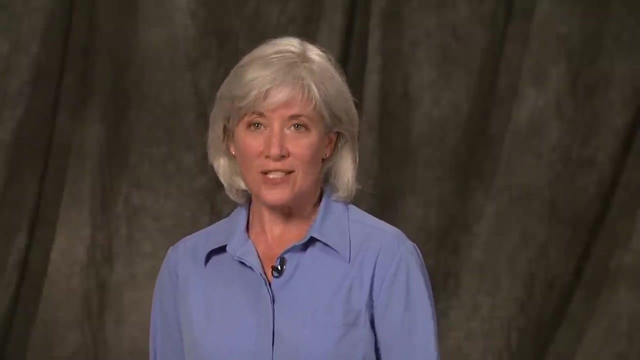 we have satisfied our body's need. In the United States, we sometimes tend to eat more protein foods than our bodies need. The trick is to eat just the right amount and not too much. We'll be talking about serving sizes later in this session. 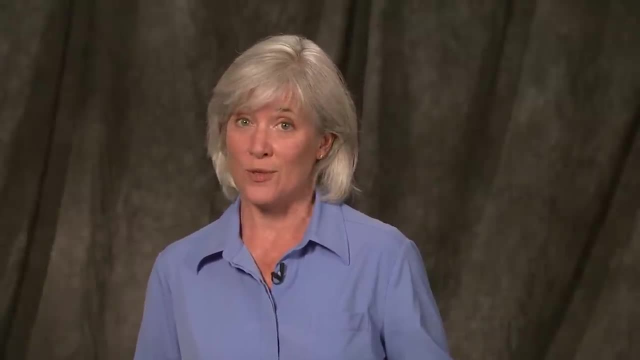 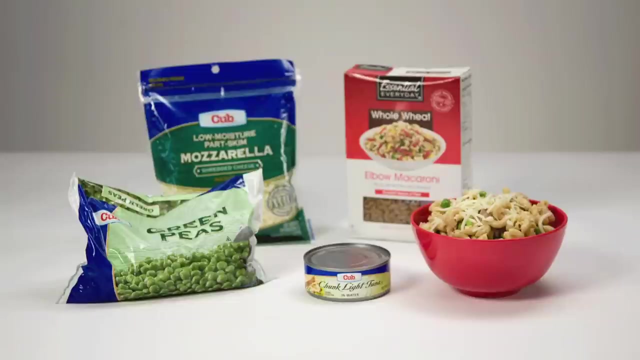 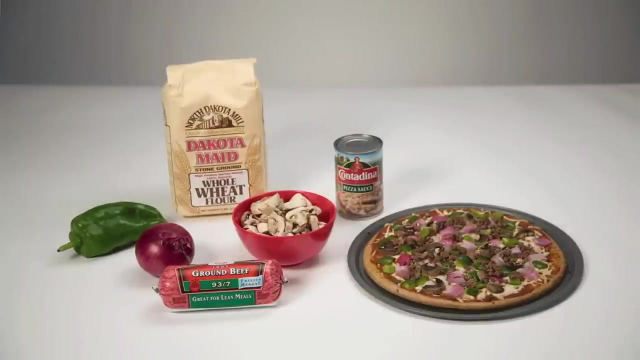 As we mentioned earlier, some foods are combination foods, like macaroni and cheese. These dishes contain foods from several food groups. This particular casserole has protein, vegetable grains and dairy. This homemade pizza is prepared with lean hamburger. 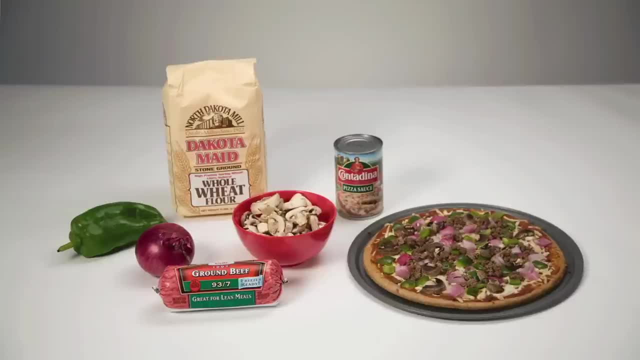 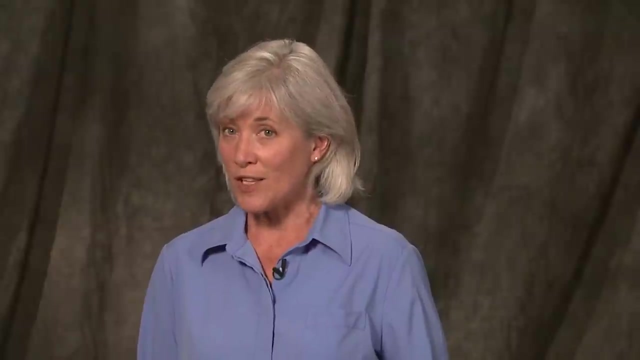 a whole-wheat crust, tomato sauce, part-skim mozzarella cheese, onions, green peppers and mushrooms. This pizza is a healthy combination food. The typical pizza we buy in restaurants or grocery stores tend to be relatively unhealthy because of the large amount of fat and sodium they contain. 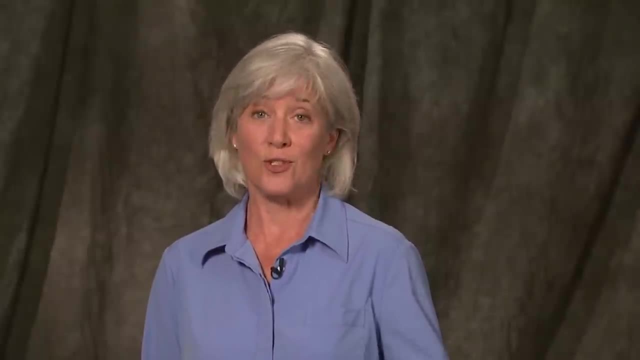 Think carefully about what you're including in the combination foods you prepare. Although combination dishes include several foods, it might not include everything you need If it doesn't make sure you add the food group that is missing to the meal to round it out. 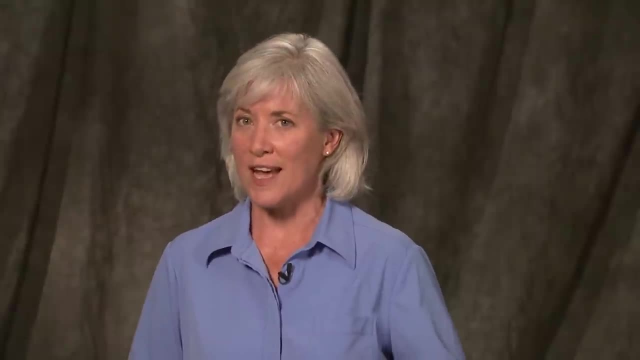 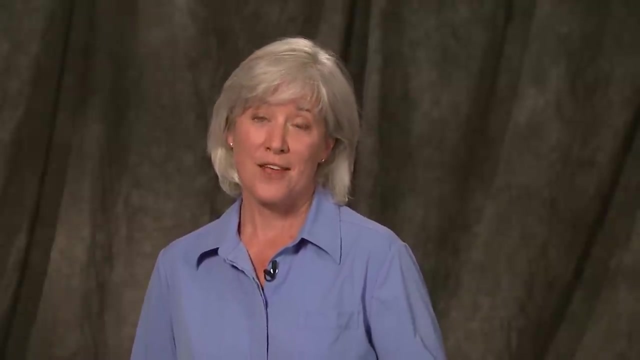 Now we need to talk about what a healthy serving size is. Sometimes it's hard to know what a healthy serving size is because there are so many different reference points. For example, this is a typical serving of pasta served in a restaurant, and this may be the amount of fat. 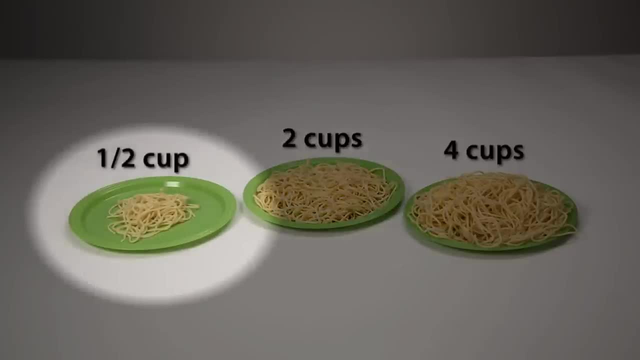 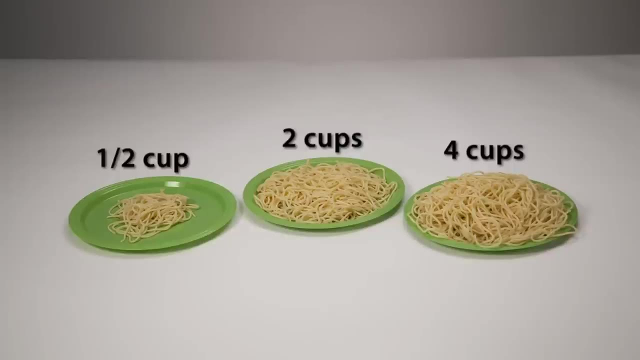 of pasta you typically put on your plate. This is actually what a healthy serving size of pasta looks like. That's quite a difference, isn't it? How do we go about making sure we're serving the right portion size? A healthy serving of food can be measured. 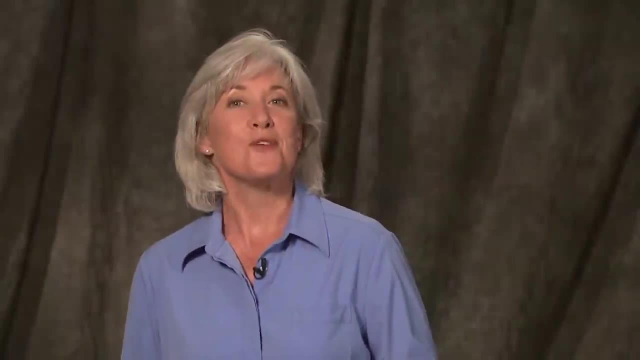 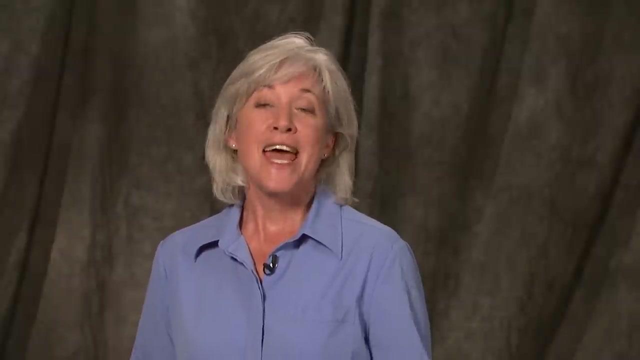 with a measuring cup or measuring spoon or something that you always have with you your hand- Parts of your hand can be a guide to measure a serving size. As we just saw, it's important to measure the amount of food that's served. 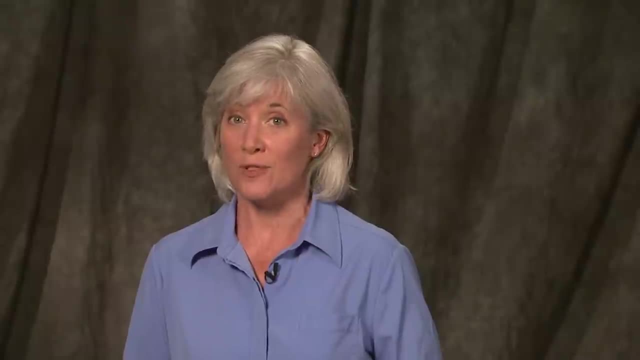 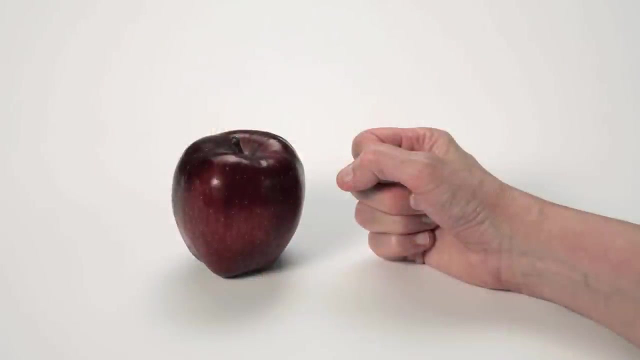 If we guess we'll likely serve too much food and too many calories to individuals, Involve the individuals you support to portion out their own foods by using these methods. Use a measuring cup or your fist to measure the following foods: Casseroles, cereal, fresh fruit. 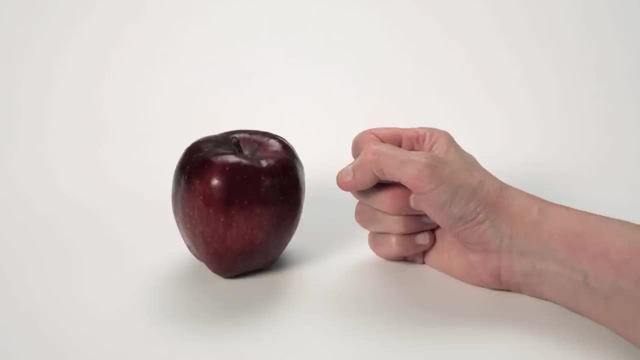 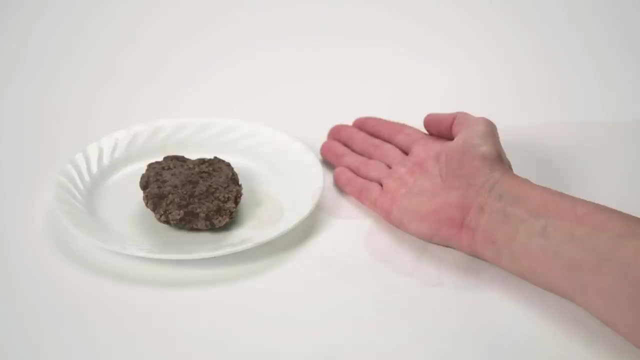 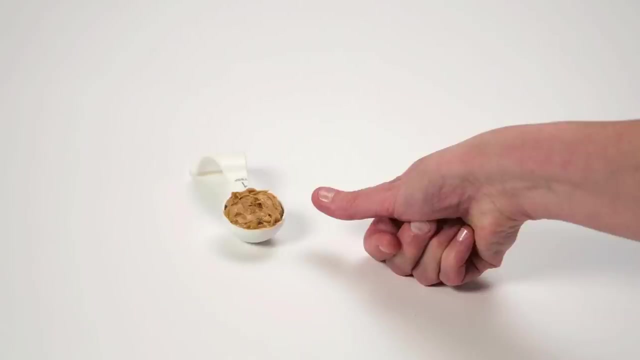 salad soup, yogurt and milk. Use the palm of your hand to measure meats such as salmon, chicken breast, pork and beef. Use a tablespoon or the size of your thumb to measure the following foods: Salad dressing, mayonnaise, oil, peanut butter. 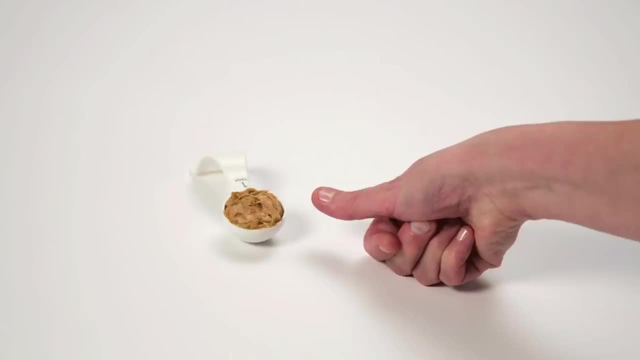 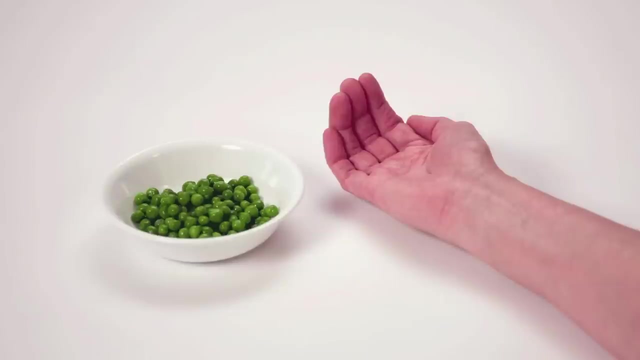 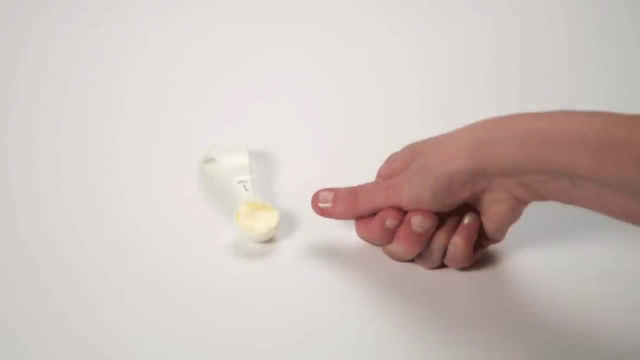 sour cream cream cheese. Use half a cup measure or your cupped hand to measure the following foods: Cereal pasta, rice cooked vegetables, mashed potatoes, cottage cheese. Use a teaspoon measure or the tip of your thumb to measure the following foods: 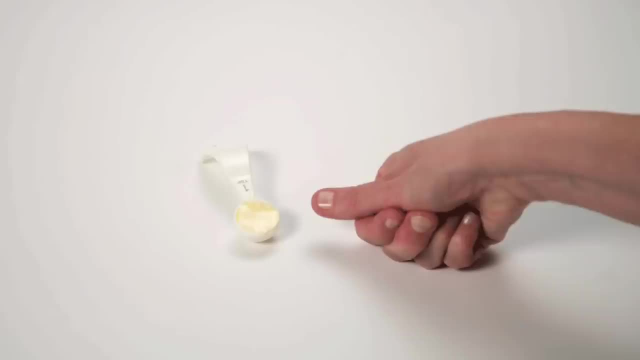 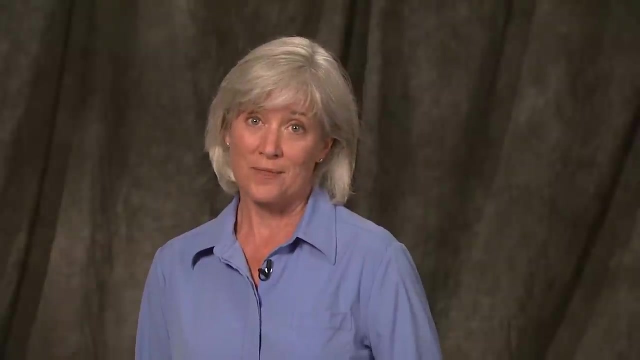 Margarine, butter, jam or jelly. Make sure you use a measuring teaspoon, not a teaspoon used for eating. This will give a more accurate measurement, Just like we've found with solid foods. we can over or underestimate how much we are drinking. 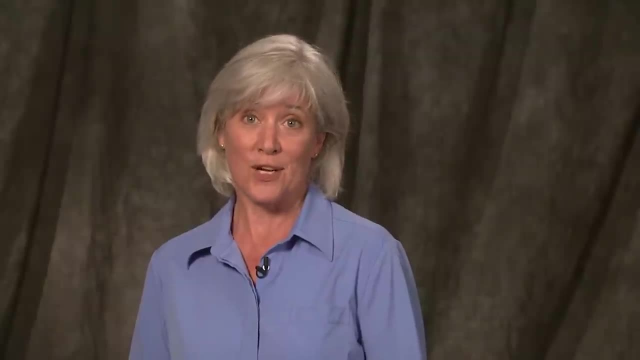 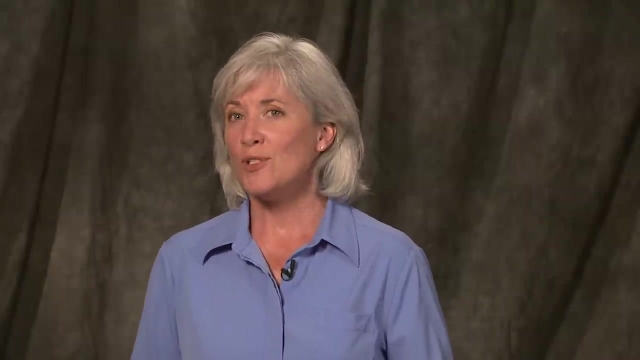 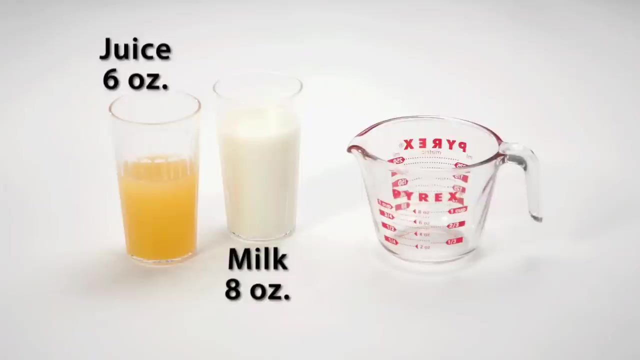 especially if we have many different sized glasses in our homes. To make sure we're getting a healthy serving size of liquids like milk or juice, it's important to know how much your glass holds. Take the glass you use most often and fill an 8-ounce measuring cup with water. 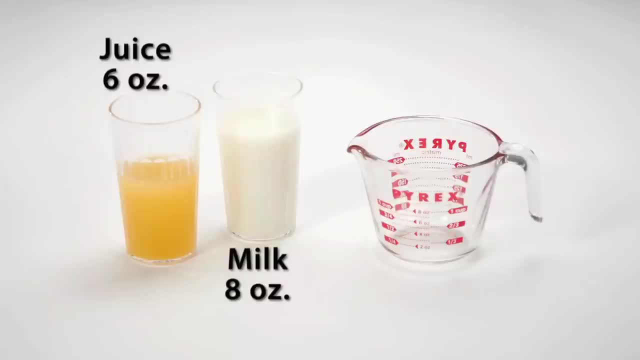 Now pour it into your glass. How much of it does it fill? This is a healthy serving of milk. Make a mental note of how full the glass should be to give an 8-ounce serving. A healthy serving of juice is 6 ounces. 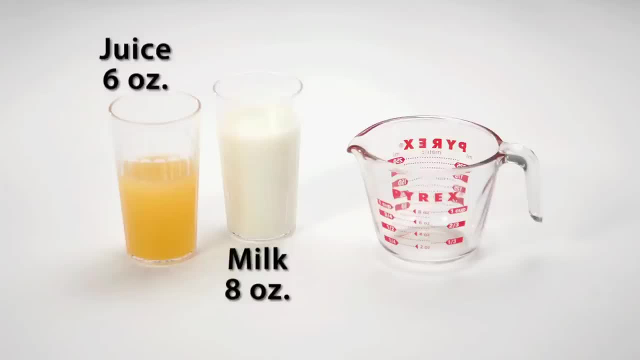 Take the glass you used most often for juice and fill a 6-ounce measuring cup with water. Pour it into your glass. How much does it fill? This is a healthy serving of juice. Make a mental note: You can't always tell by looking at a glass. 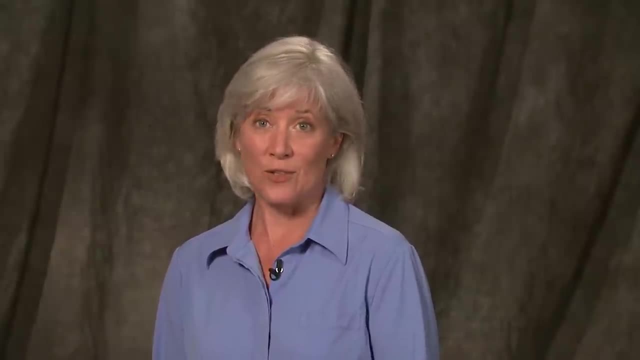 how much it holds. Tall skinny glasses usually hold less and short wide glasses usually hold more. But the best bet is to measure before you pour. Similarly, we can't always easily tell by looking at our plates how much food we actually have. 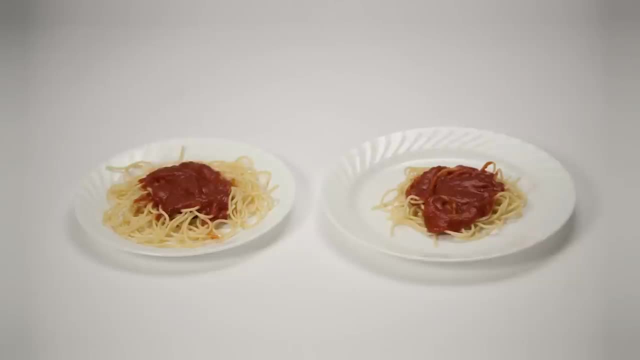 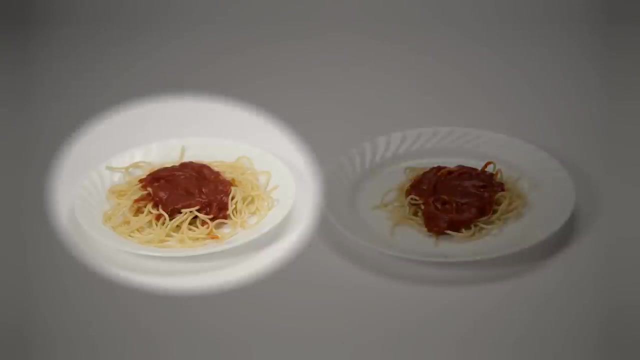 Each of these plates has the same amount of food on it. As you can see, if you eat from a smaller plate, the food portion looks bigger. The size of your plate really does matter when deciding how much food you would actually put on your plate. 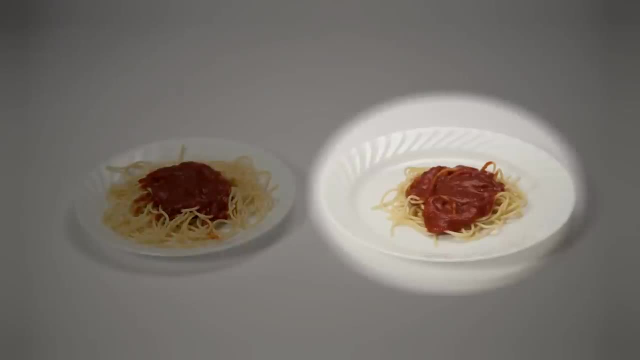 For example, on a large plate, a healthy serving size of pasta, looks like you don't have much to eat. If you place the same amount of pasta on a smaller plate, it looks like you have the right amount. Studies show that people who eat from smaller plates. 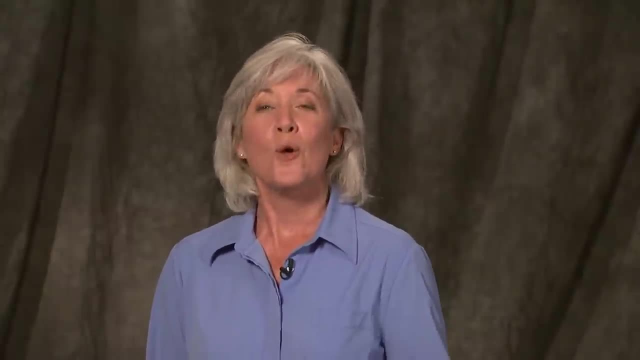 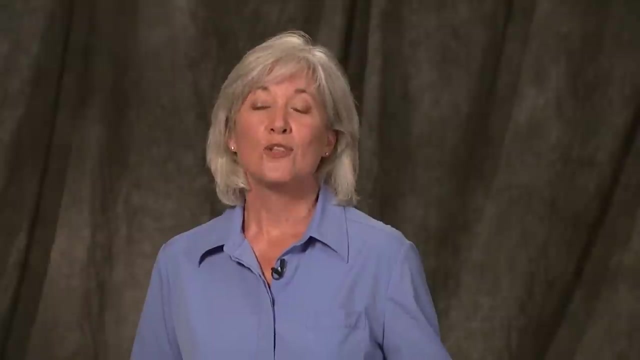 actually eat less. We eat with our eyes first. If you don't see enough food on your plate, you're going to think you need more, So reach for the smaller plates first. Here's a summary of the main points I've made. 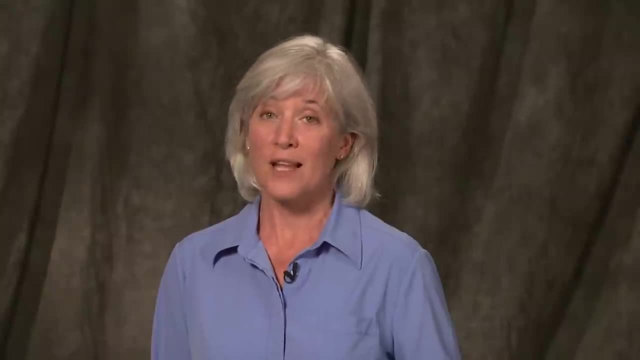 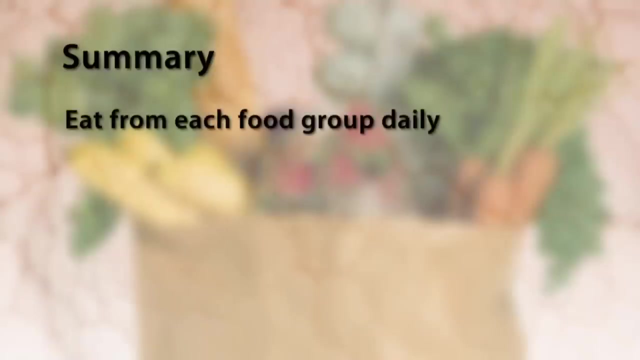 Follow the balanced daily plate to serve the right balance of foods individuals need each and every day. We all need to eat from each of the food groups every day to be healthy. Fruits, vegetables and grains should be the foundation of our diet.